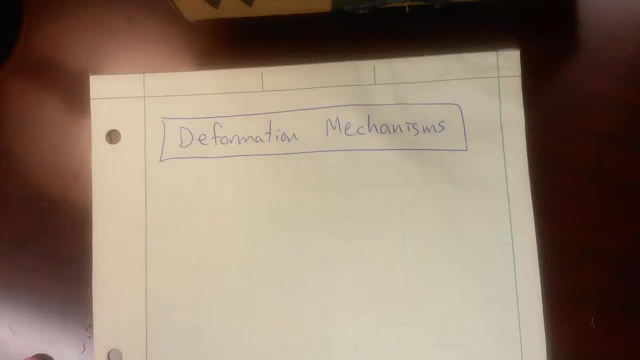 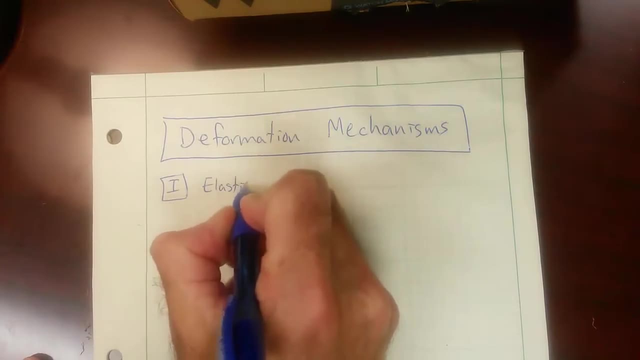 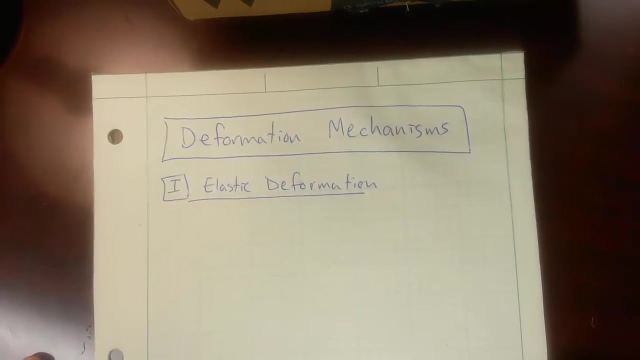 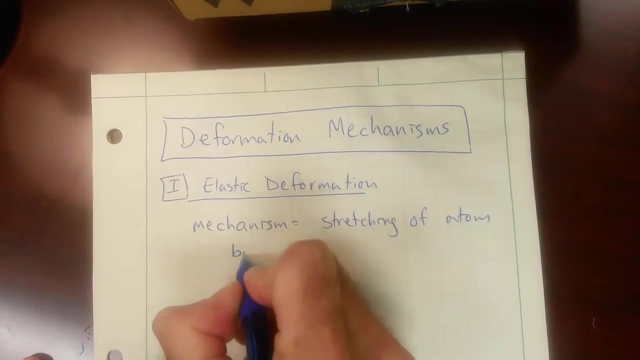 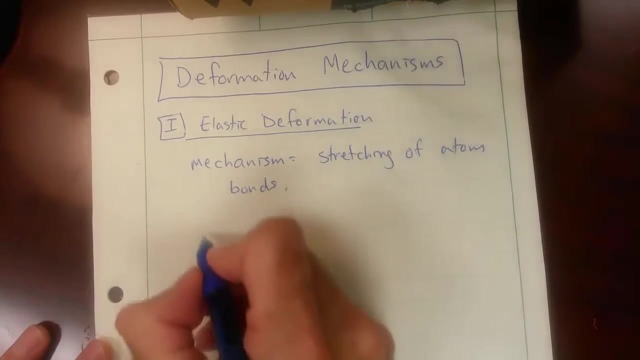 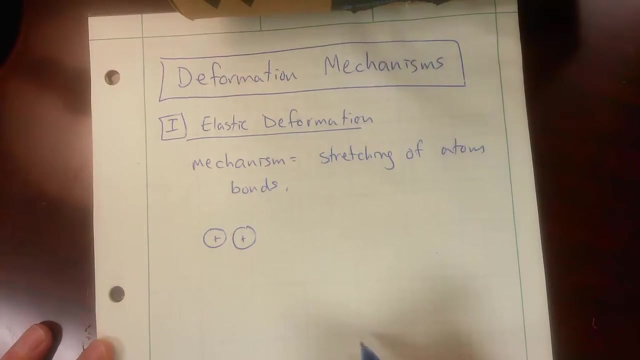 do metals deform? How do the atoms rearrange themselves under stress? First we'll talk about elastic deformation. In elastic deformation, the mechanism of deformation is the stretching of atomic bonds. The mechanism is the stretching of atomic bonds. So if we have two atoms, then separated by some distance, a, and we apply a force, the 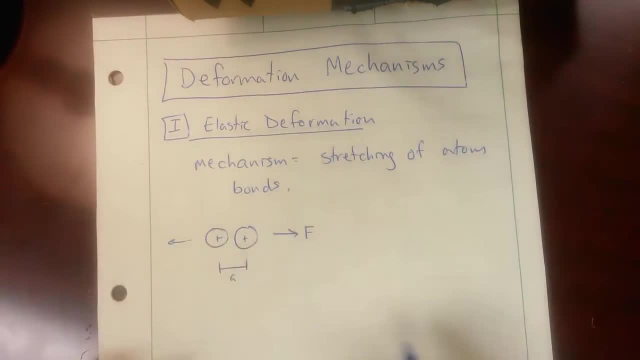 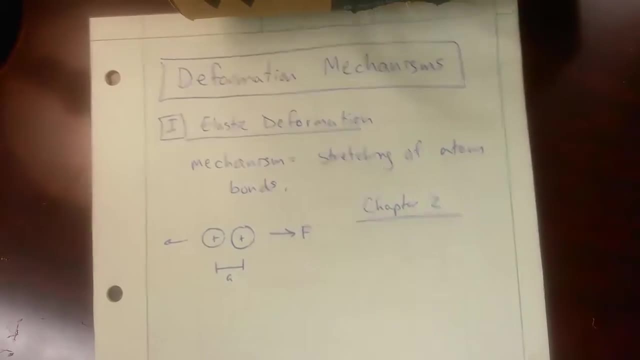 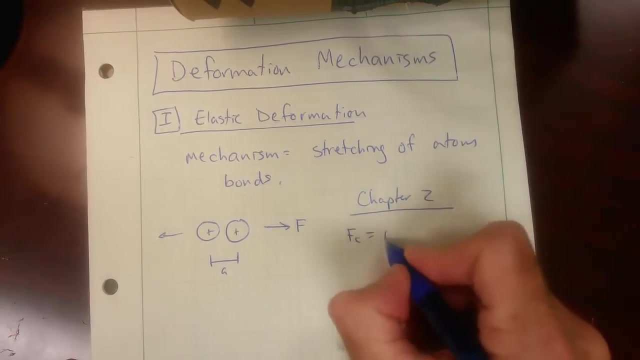 atoms will move farther apart And when we remove that force they will come back together. If you will recall from Chapter 2 of the Shackelford textbook, the forces between the atoms is made up of a coulombic attractive force. Fc is the attractive force. 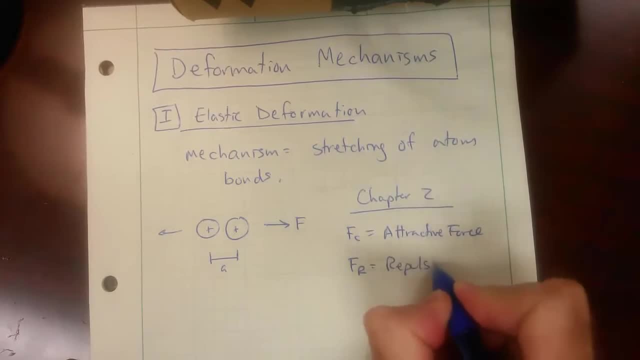 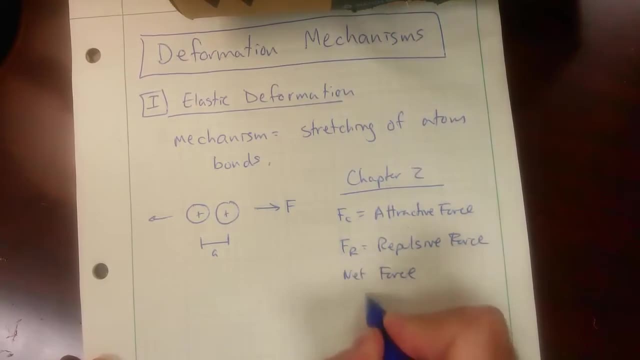 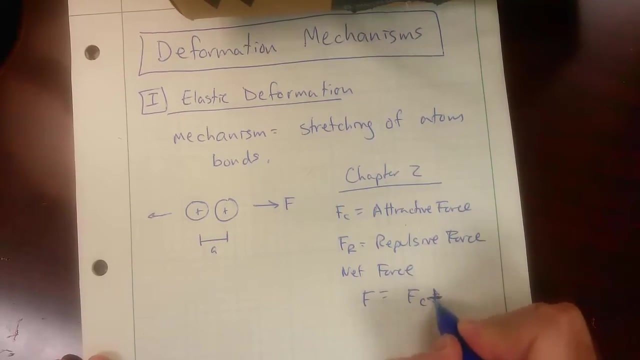 Fr is a repulsive force And the net force is F, which is just the sum of the coulombic attractive force plus the repulsive force. In Chapter 2, there was a picture, Figure 2.7.. It's hard to read that so I'm going to redraw it here, but there's some. 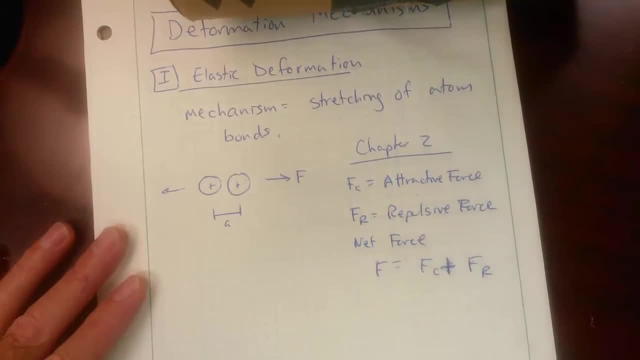 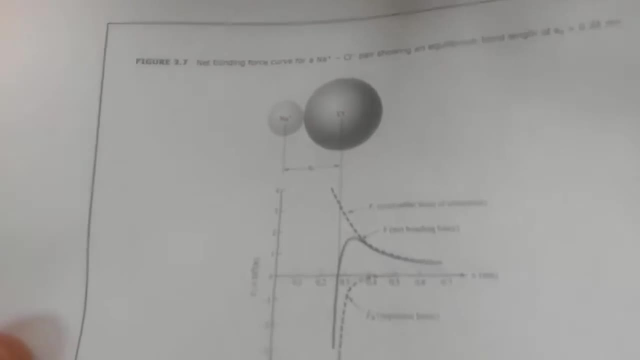 good literature in this common barracks in S победa bque Mexico. они об geographicar и хлоп Buenoslene, Kansas. The daughters are going to have kids And the children will have a baby boy with a chance to看. ward to their chances of pumpkin and tusk? are they going to make them freeze or wake up from the heat? Meatballées par mexicanos e 1600eapostas. dunei观 한국ич的人. So I'm going to redraw it here. 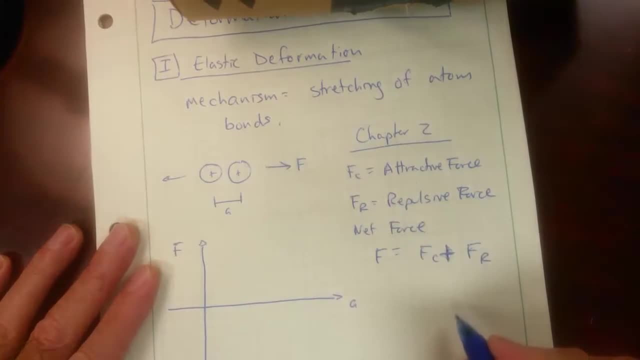 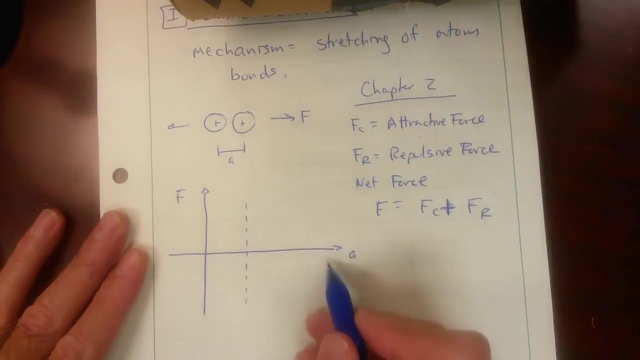 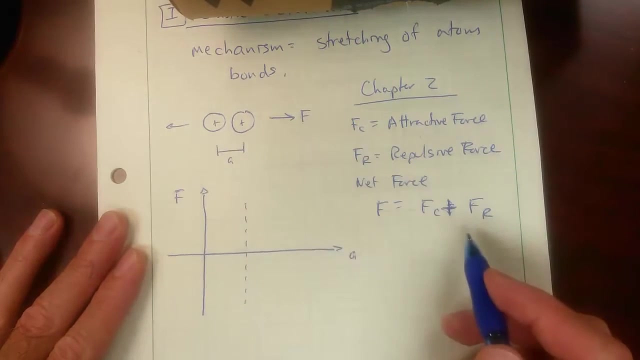 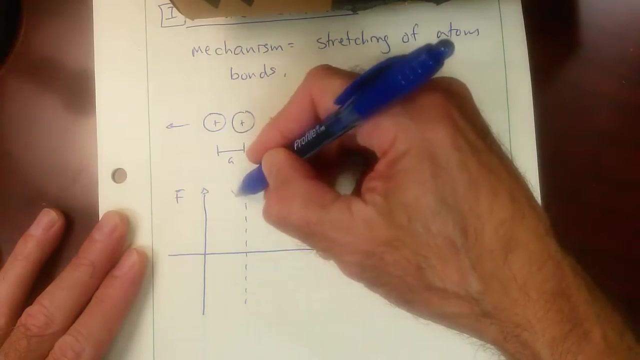 Force versus position A And I'm going to draw a dotted line about one-third of the way out on the A-axis. So the attractive force increases as the atoms get closer together and it decreases as the spacing increases. So our attractive force curve looks something like that: 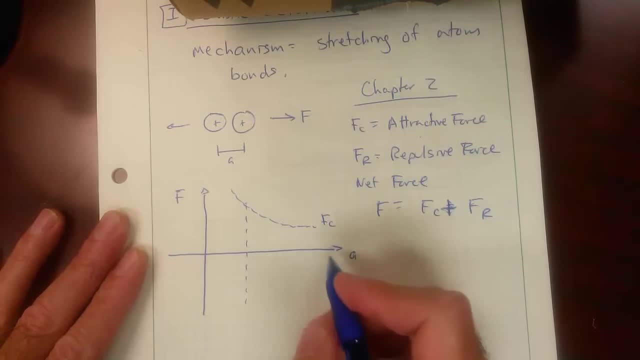 The repulsive force becomes greater in a repulsive sense or in a negative sense, as we push the atoms together. So we have a curve that looks like that for the repulsive force, And when you add these two together you get a curve that's shaped. 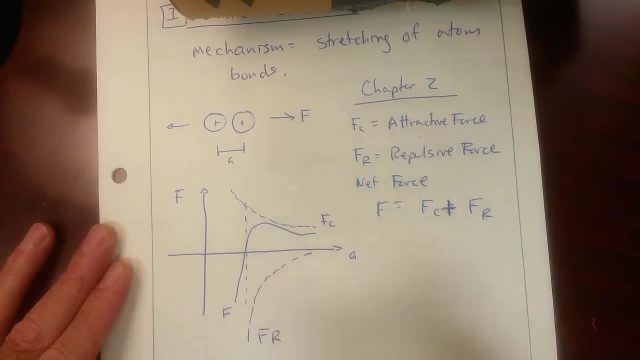 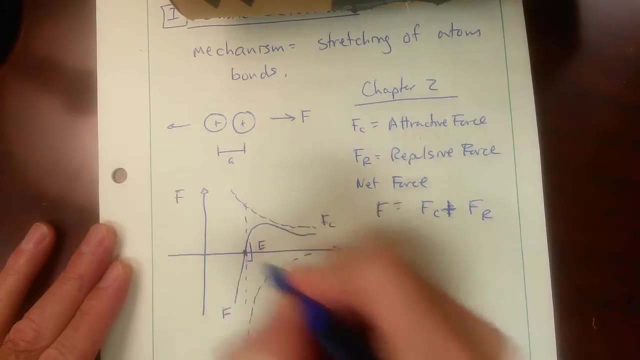 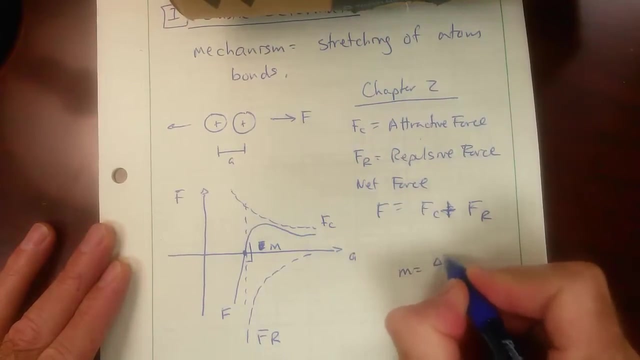 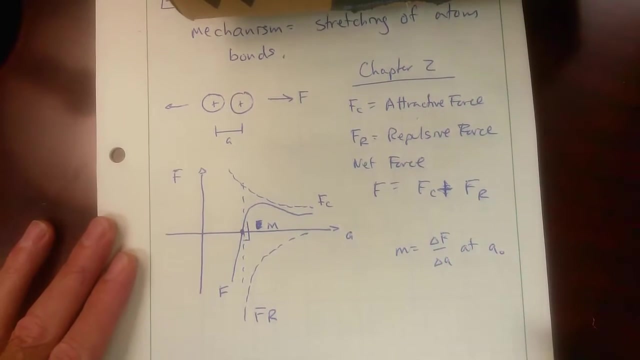 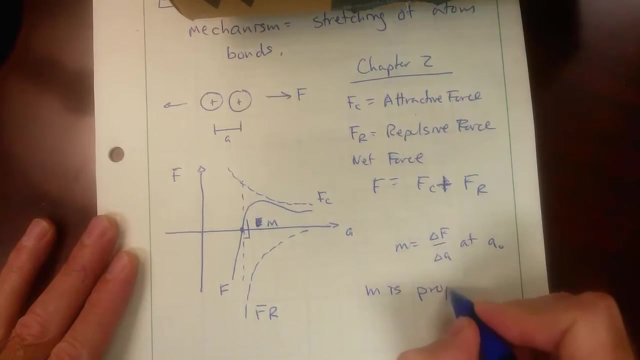 kind of like that which is the net force. So right around here, where the force is zero is our equilibrium distance And right there the slope of the F-A curve is delta F over delta A at the equilibrium position A-zero And M is proportional to the elastic modulus. 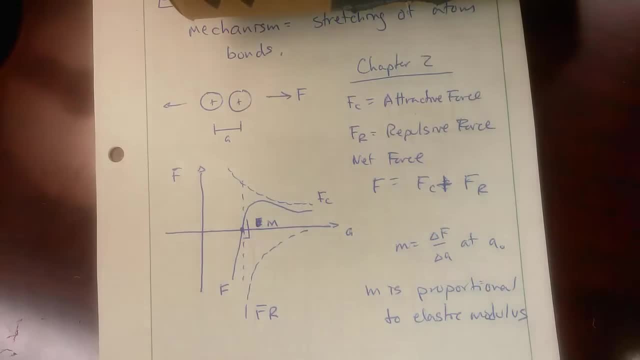 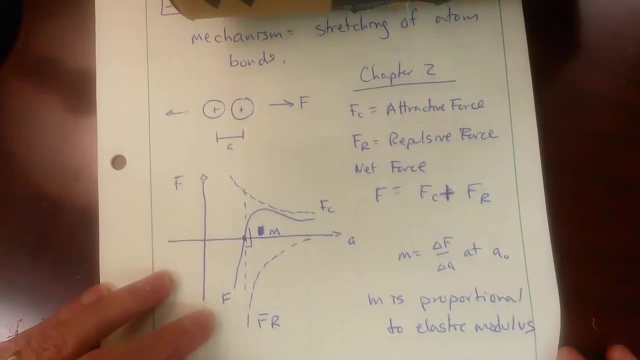 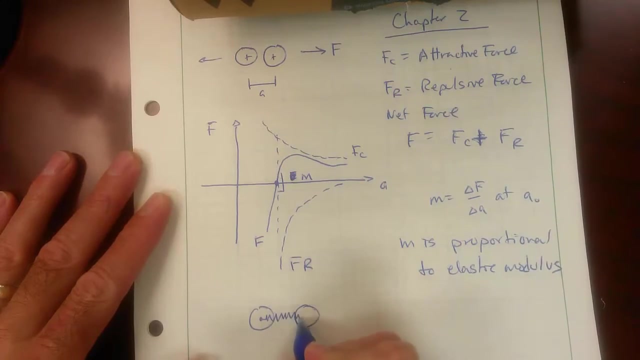 M is proportional to the elastic modulus. So that's pretty simple Things. uh the stretch. you can almost see us think of the elastic deformation acting like a spring between two spheres where, if we pull them apart, the spring wants to pull them back together As we. 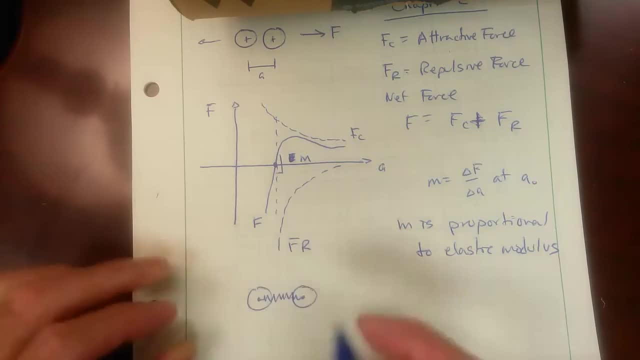 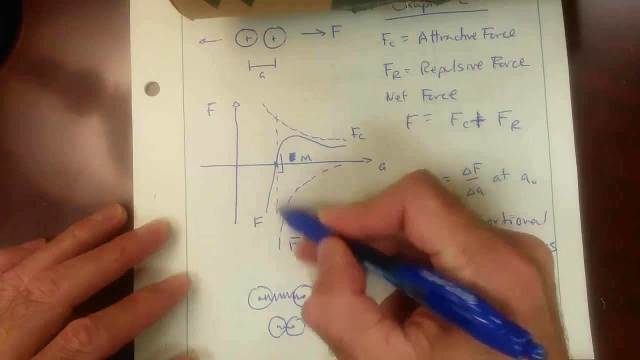 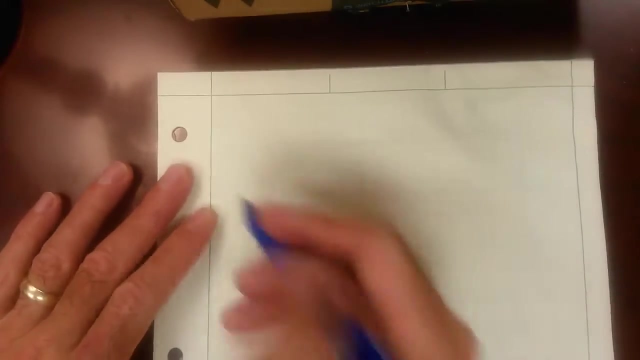 compress the spring, the resistance increases until we get to a point where the two spheres are actually touching, at which case the force becomes infinitely large to move them any closer together, which is why this curve drops sort of asymptotically. Things I think are a little more interesting when we talk about plastic. 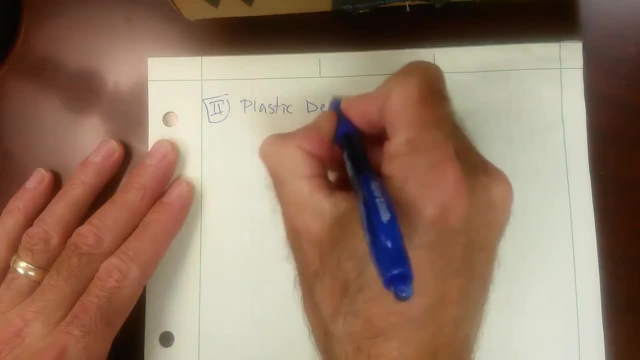 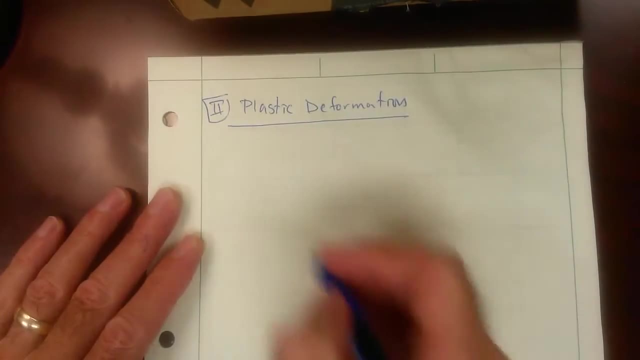 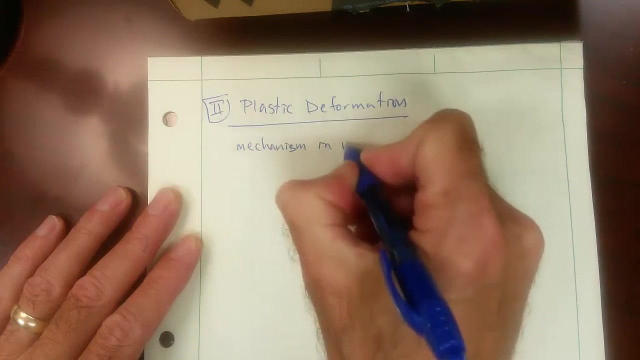 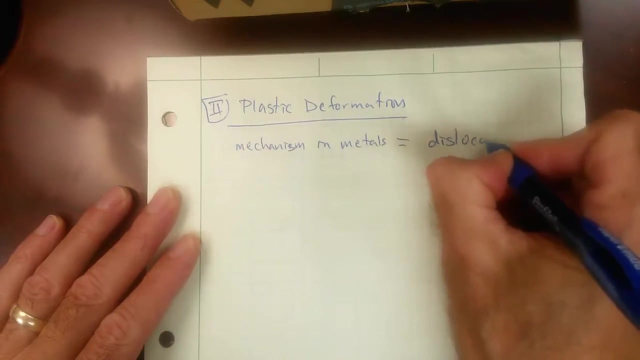 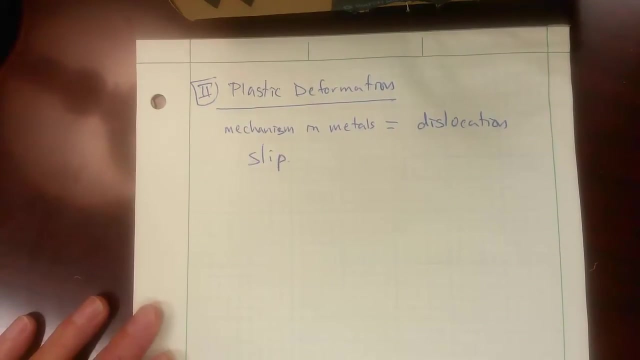 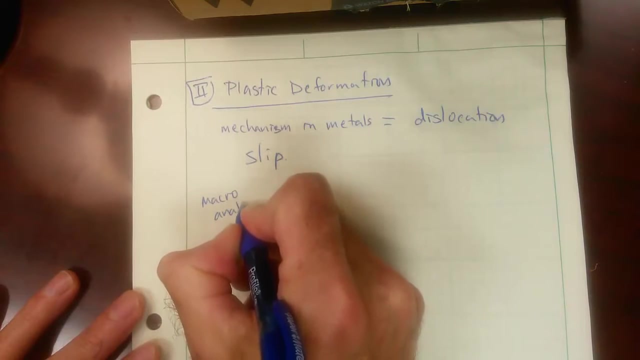 deformation. Section 2 is plastic deformation, And the mechanism of plastic deformation in metals is dislocation slip. Dislocation slip- Now it's kind of a weird thing to understand. So I'm going to give a macro analogy And I'm going to talk about a rain tarp. 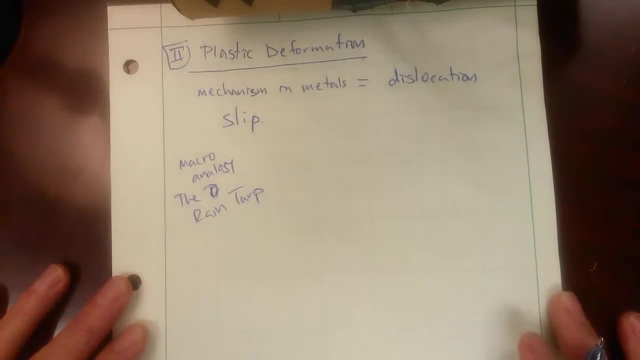 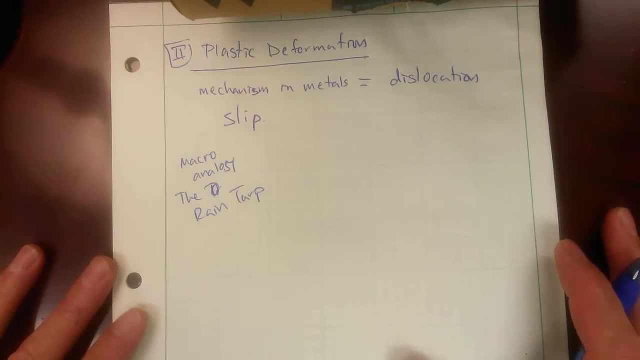 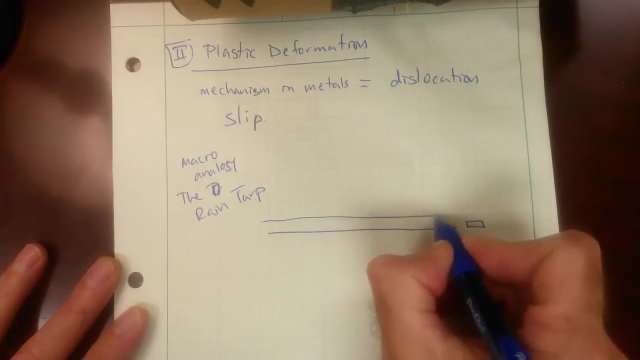 So I was at a minor league baseball game and it started to rain And some dudes came out with a big piece of plastic to cover up the field. And here's the field, and let's say this is third base. And what they did was, when they rolled the tarp out, they didn't cover third base. 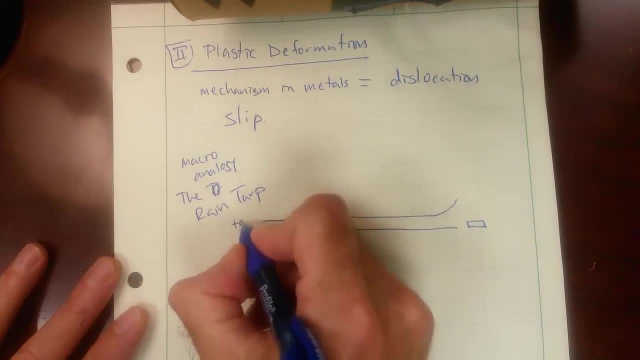 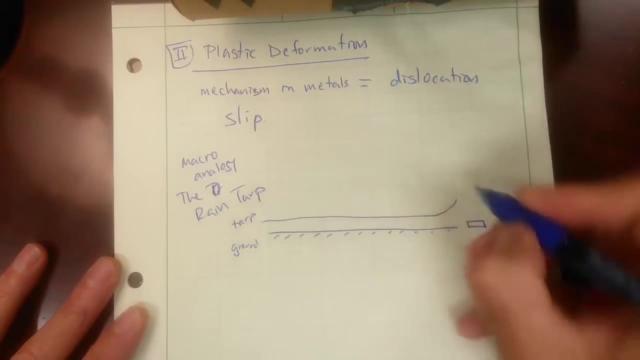 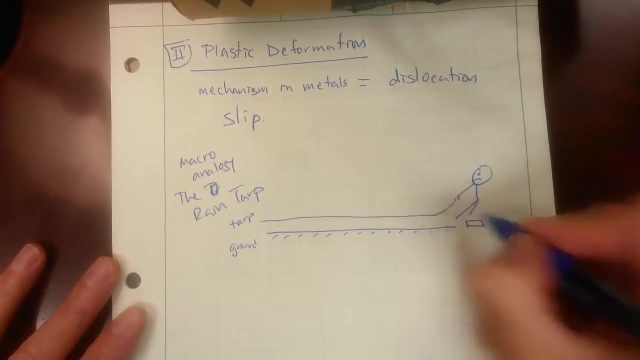 So it didn't make it all the way there. So this is the tarp and this is the ground, And so this dude was standing there And he was pulling as hard as he could and could not get that tarp to move. 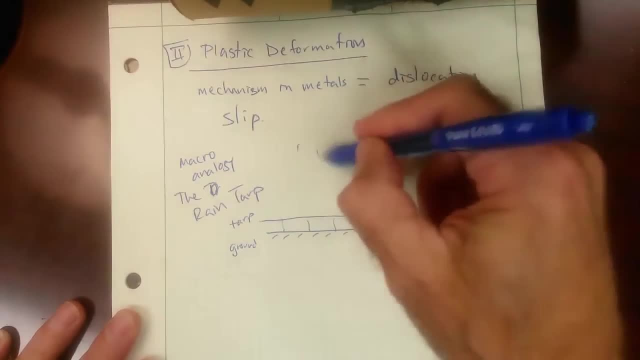 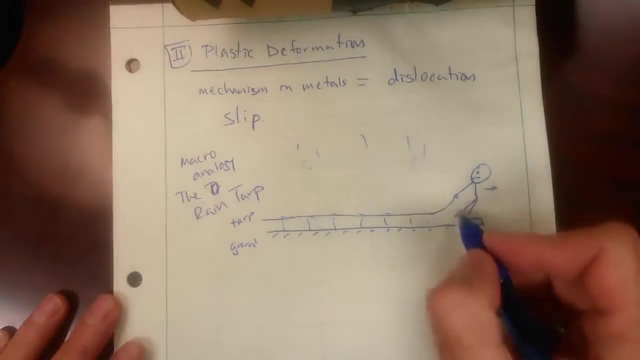 because it was touching the ground all along here And it was raining. And the more it rained, the heavier the tarp got and the more futile it seemed for this dude to be able to pull the entire tarp and have it slide along the ground. 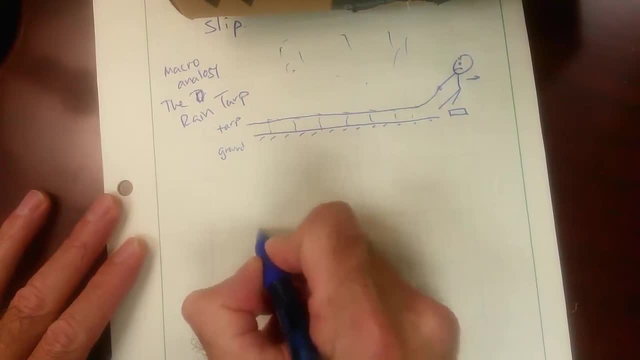 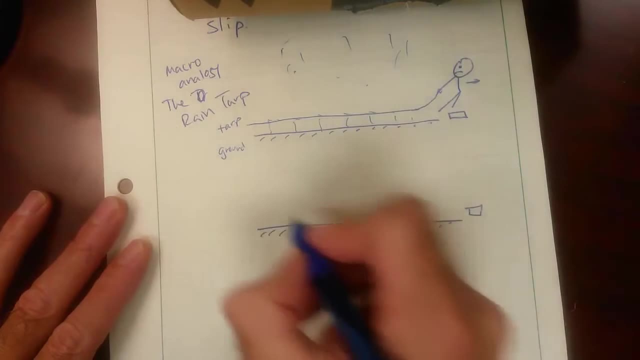 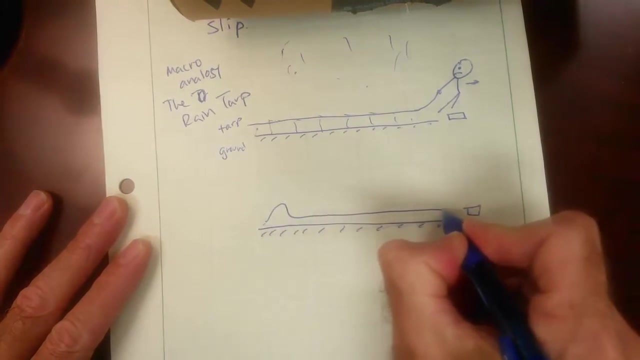 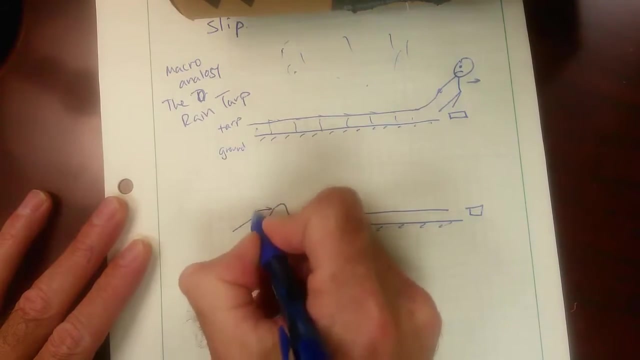 Well, somebody who was Somebody who was smart came out and introduced the dislocation And there's third base, And what they did was they picked up this end of the tarp And they were able to just push that dislocation or that. 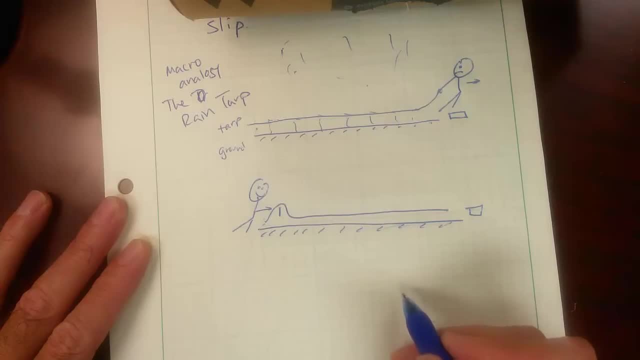 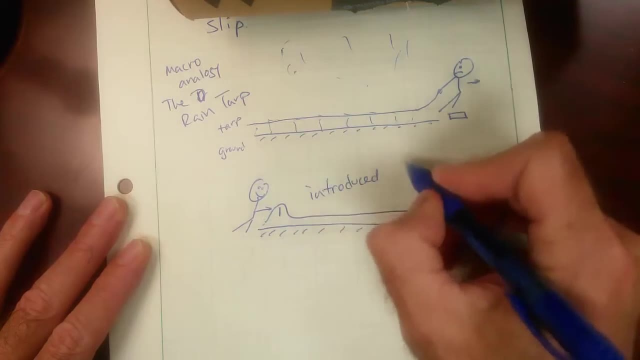 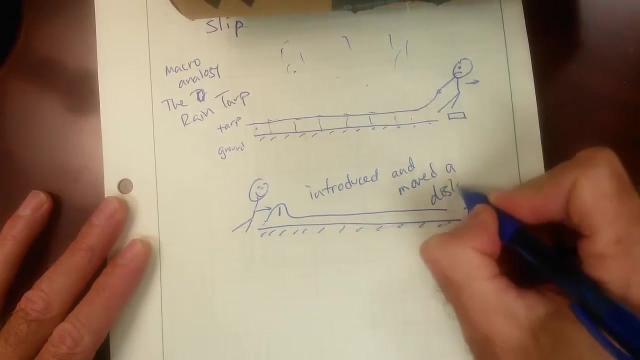 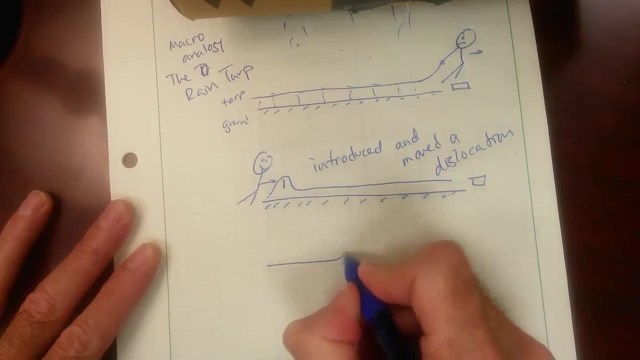 Yeah, So they were able to just push that dislocation along the length of the tarp. So what they did here was they introduced and moved a dislocation, So a little while later, as he was pushing it along, let's see, let me get this right. 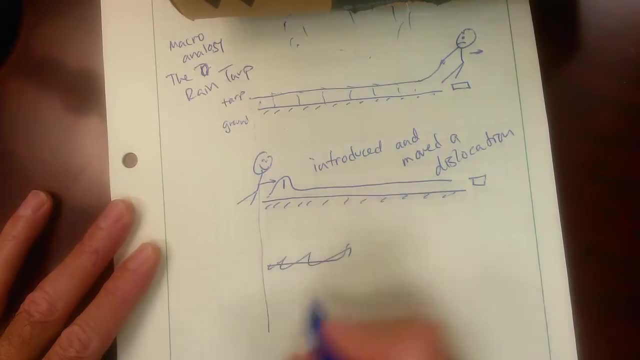 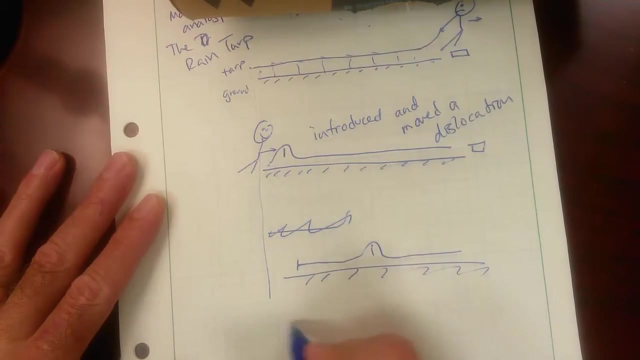 So this is where it started. So a little while later we introduced the dislocation. That end of the tarp had moved, There was a dislocation still hadn't reached the end yet, and eventually the dislocation was moved all the way to the end, at which point it popped out and we were able to cover.